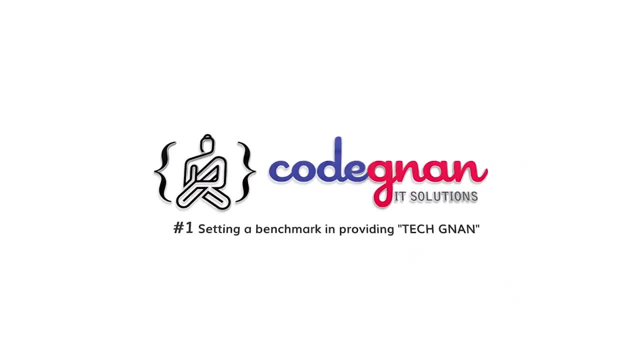 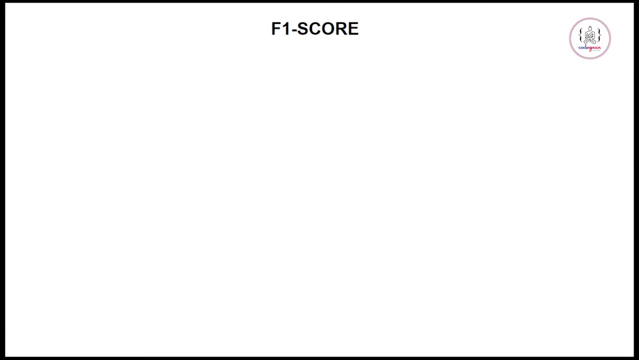 Hello everyone and welcome. In this video we are going to see what is F1 score. So before moving forward, make sure that you have watched the confusion matrix video on our YouTube channel. So here we are going to also consider an example, so it is better to understand anything. 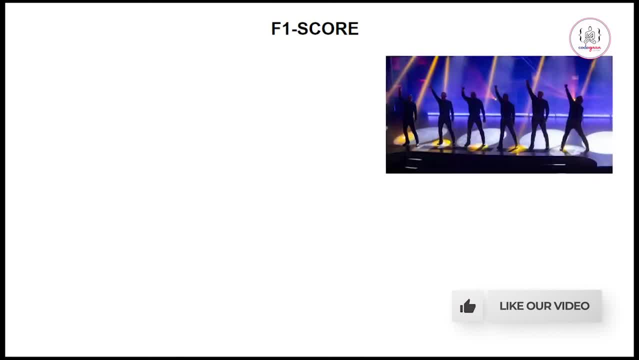 with example, right? So here let's say you are running a show and you want to find out whether the people are going to like your show or not. So you did some kind of survey and you find out out of this 10- sorry, 1000 people, you find that 999 does not like the show and only 10 people. 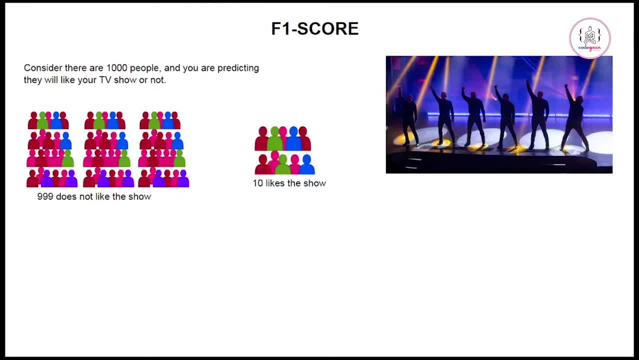 like the show, Right. So here, if you say that nobody likes the show, then you are going to have a high accuracy score- that is 99 percent, right? So here, by simply simply saying that no one likes the show, you have 99 percent of accuracy, but you are not able to identify those 1 percent. 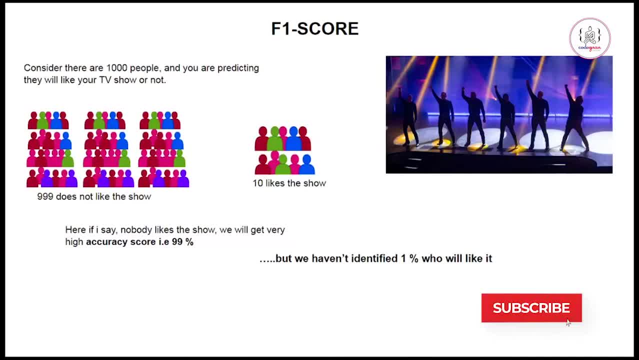 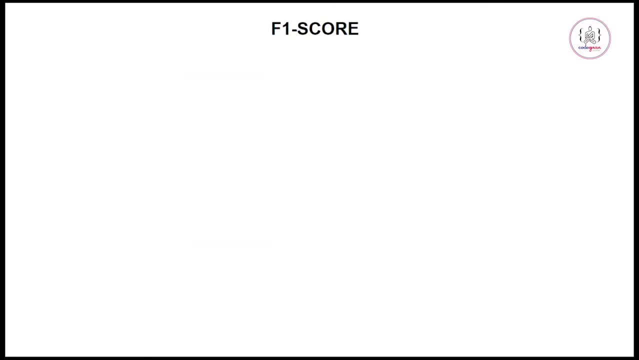 people who are going to like your show Right, And for that reason we cannot use only this accuracy score. For that reason we came up with precision and recall. So let's see what is precision and recall. So precision is how accurate you are. 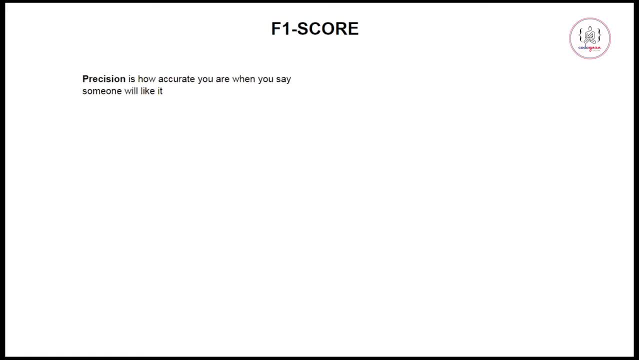 when you say someone will like it, Right. So here, if you say that eight people like the show and out of which only six actually liked your show, then your precision is 75 percent Right. And recall is how good you are at identifying people who actually like it. 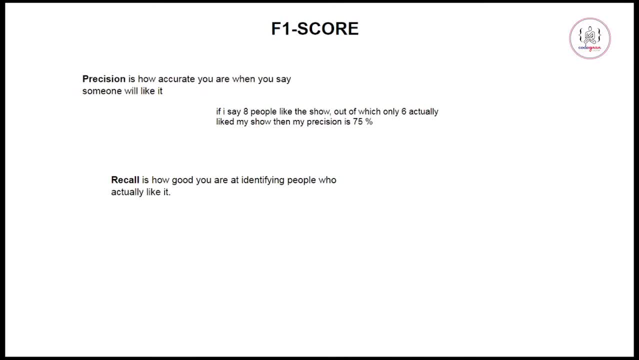 So we have seen that 10 people are there who like our show, and out of those 10 people, we are able to correctly identify only six or more people who like our show, Right. So we came up with a record of 80 percent of them. So here, Oh and recall, is 60 percent Right. 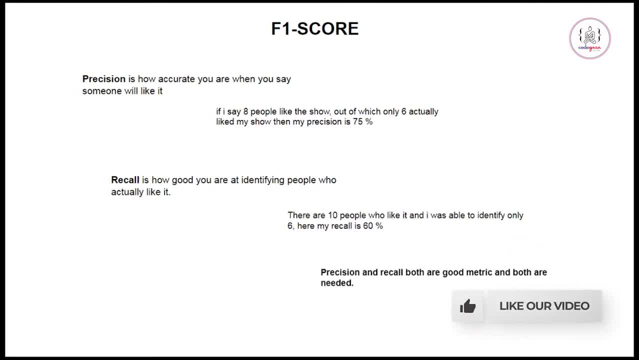 So precision and recall: both are good metric and both are needed. So why do we came up with this F1 score so you will see that in our next slide, Let's see here. So let's consider this scenario where I say: nobody likes the show. 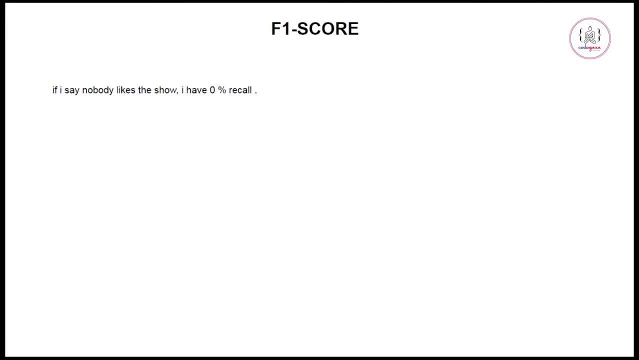 All right, no one likes the so, so we are not able to identify those 1% people who are going to like our so right, so I have 0% recall here and it is bad, right, but if I say everyone likes the, so I have 100% recall but only 1% precision, which is bad again. now we have seen that we have when 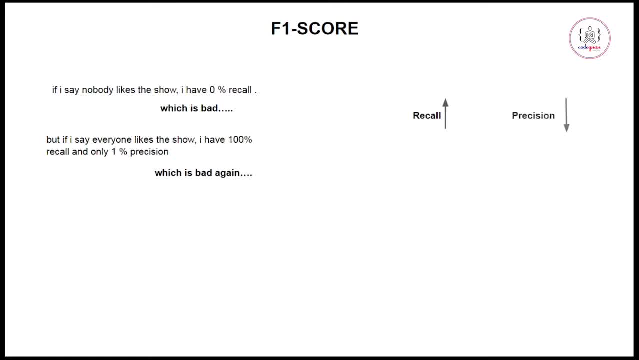 we are increasing this recall, our precision is going down right, and if you increase this precision, your recall will go down. so there is this trade-off between recall and recall. so I have 100% recall but only 1% precision, which is bad. again now we have seen that we have. 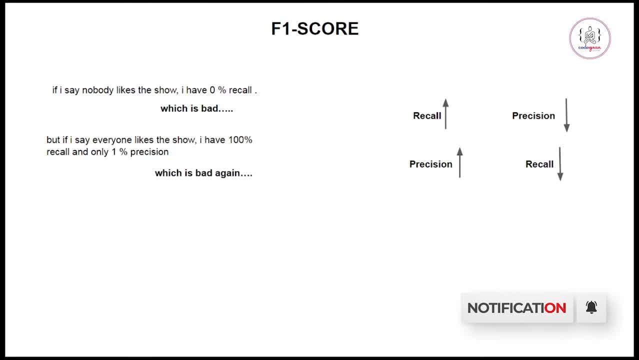 precision. now, how to consider which value do we settle in right, which value of recall and which value of precision? so now you'll be scratching your head right. so what value should you consider? how about if we take this precision and recall and we average them out? so let's see that and let's consider this example here, which is everyone. 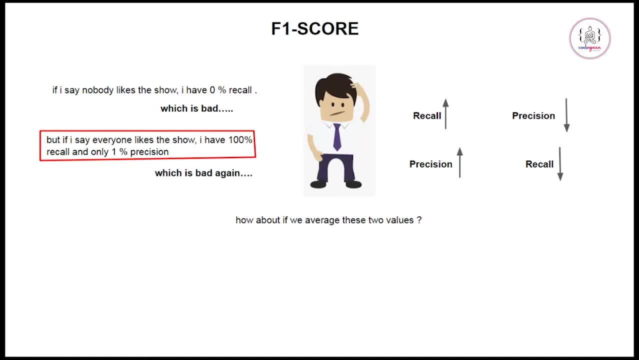 likes the so and we have 100% recall and only 1% precision. if we average this, it is going to be 100 plus 1 by 2, right, and which is equals to 50.5. but the average of precision and recall here is: 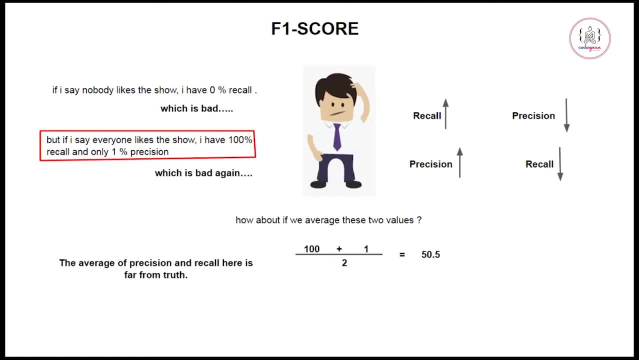 far from the truth. right, you only have 100% recall, but the precision is 1%, so this does not reflect the right metric. so simply averaging precision and recall is not enough here. that's why we use harmonic mean for precision and recall, right. so here, if you use 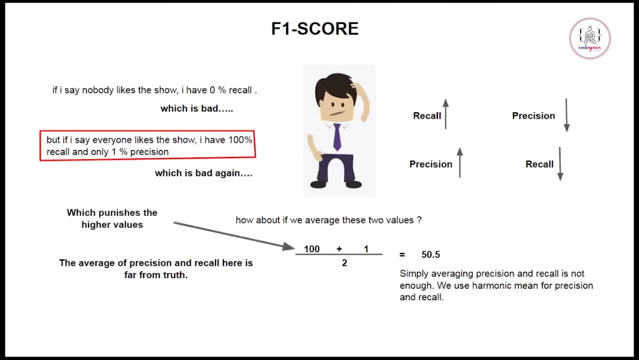 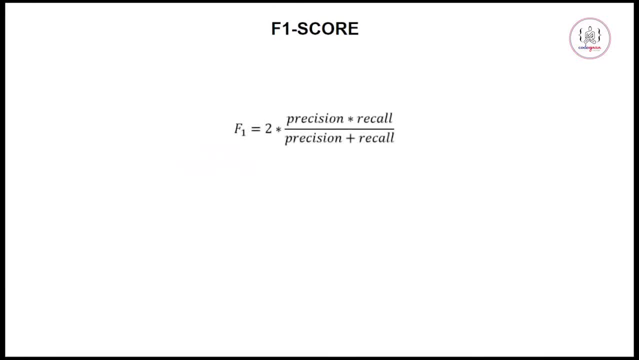 harmonic mean it is going to punish this higher values, and you will see that in our next slide here. so here, f1 score is calculated by this formula, which is equals to 2: X precision, X recall divided by precision plus recall. so this is your f1 score. 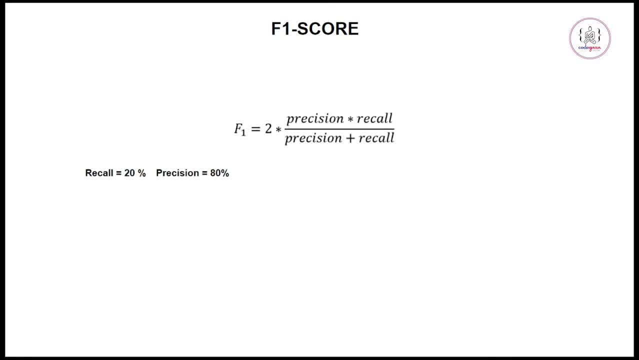 Now let's consider this example here, where we have this 20% precision- sorry, 20% recall and 80% recall precision here, and if we cap, put this value in this formula, we are going to get 0.32 right and here, if you see, the recall was 20 percent, precision was 80 percent. but our value that we have, 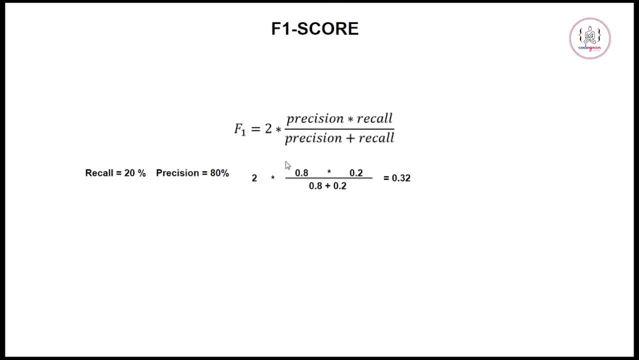 calculated, that is 0.32 is close to recall. here lower value, right. so here we are punishing this: higher values again you have. let's consider another example where we have 10 percent of recall and 90 percent of precision. so here it is going to give you 0.12 again. it is closer to your lower. 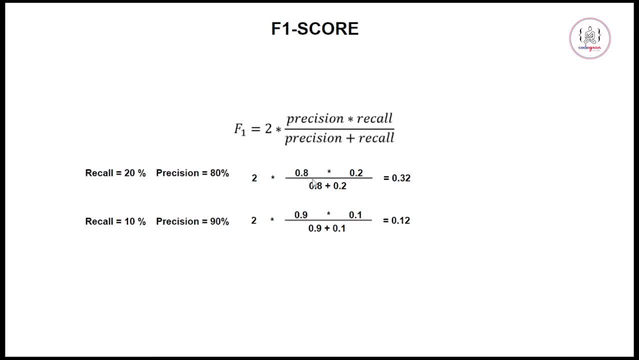 value that is your recall. here, right again, you are punishing this higher value. so this is why we use f1 score and we calculate the harmonic mean of precision and recall, and we use this f1 score in combination with other matrix, so it is very rarely used in machine learning.